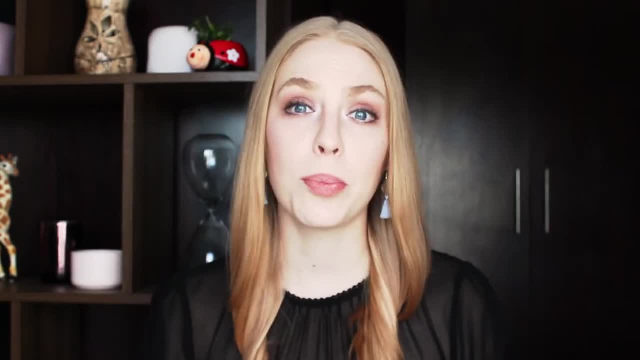 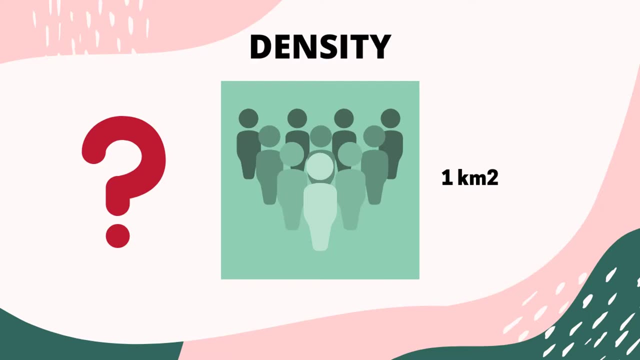 of measurement for area With population density. we are basically looking at how many people there are within Superior Regional Dep忑 ie48.. one little area. The more people there are in that defined area means that there is going to be a higher population density, and the fewer people there are in that defined area means that there's. 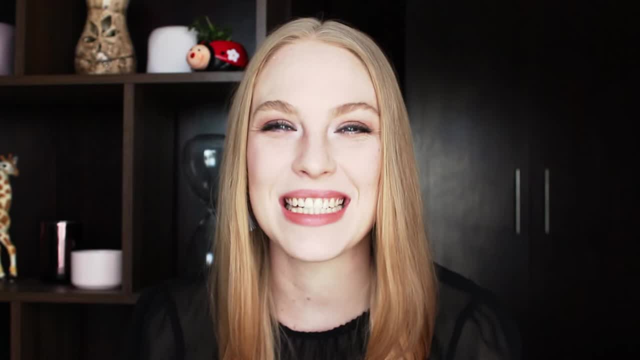 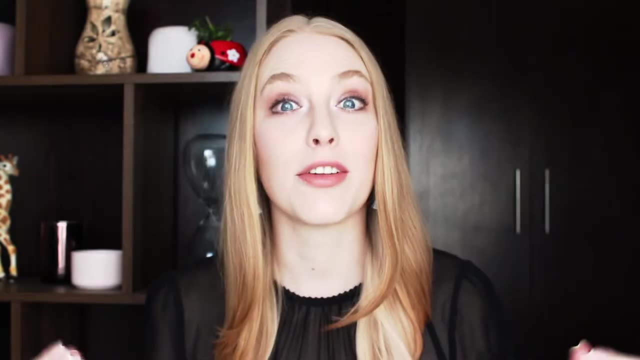 going to be a lower population density, but we'll get to that in just a moment. Let's first have a look at the different types of population distribution that exist. The first type of population distribution that we will look at is dispersed, also known as scattered Dispersed. 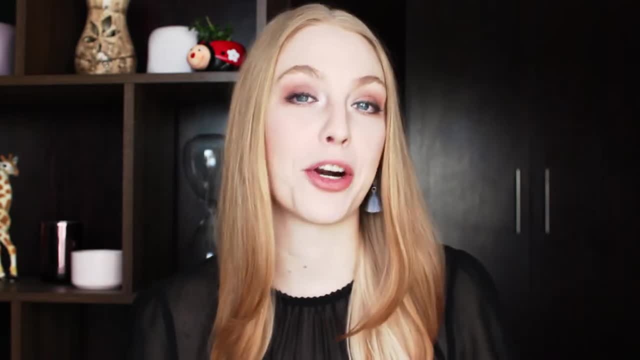 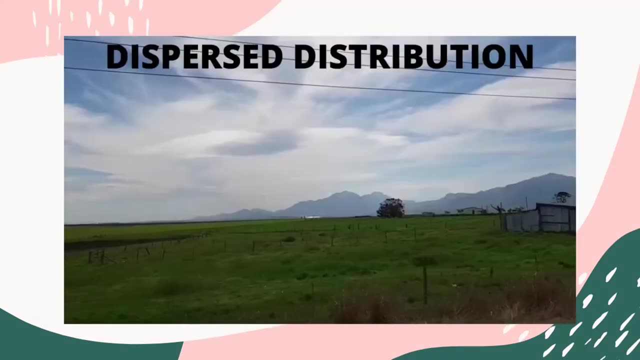 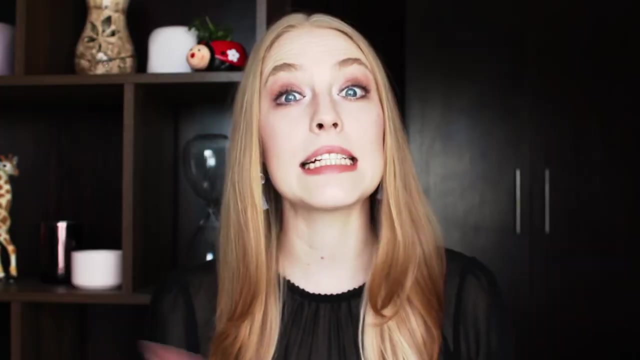 population distribution is when people live very far apart from each other, and this is very common in rural areas, especially farmlands. So each farmer and his family will have their own house and their own plot of land, and it is very far from all the other farmers. The next type of 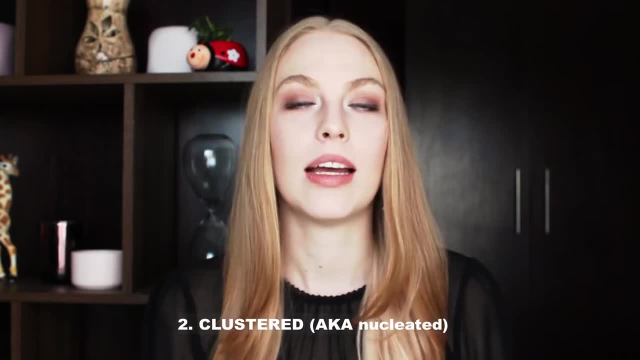 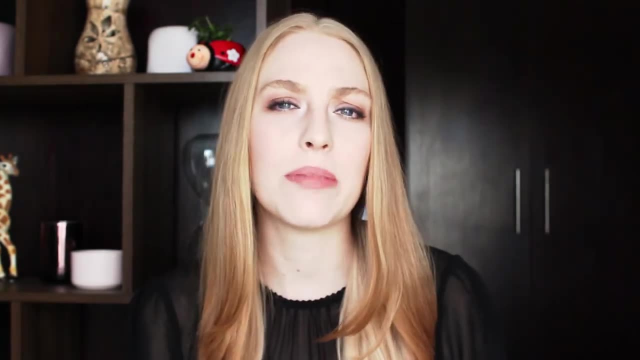 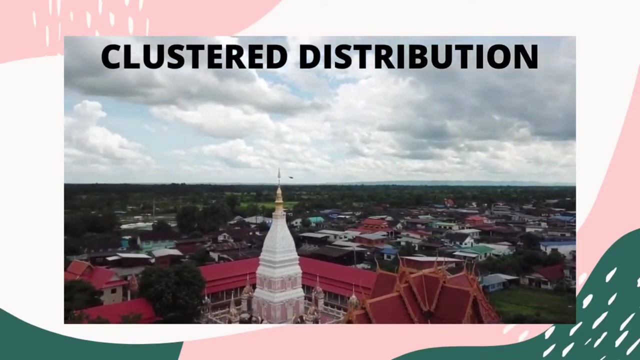 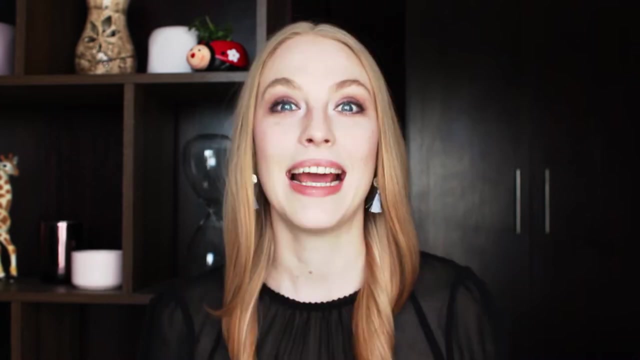 population distribution is clustered. Another name for clustered can also be nucleated With clustered population distribution. houses and buildings are built fairly close together, and they are often built around a central point such as a church. Any new towns that are planned and developed nowadays tend to be built in this clustered fashion. Our third and 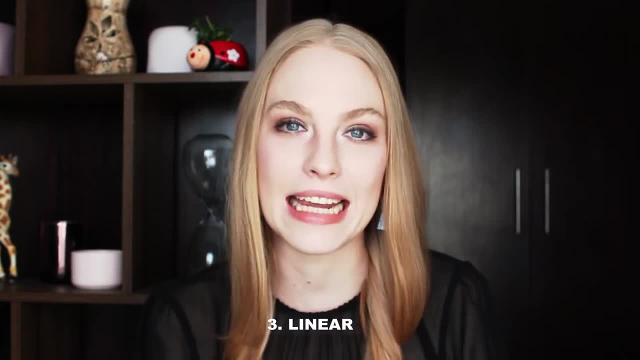 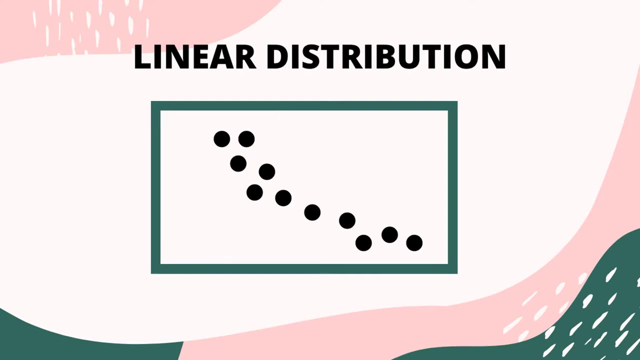 final type of population distribution is called linear. Linear population distribution happens when houses or buildings are built along a certain feature, such as a shoreline or a river, or even a road. Now that we understand the different types of population distribution, let's look at the. 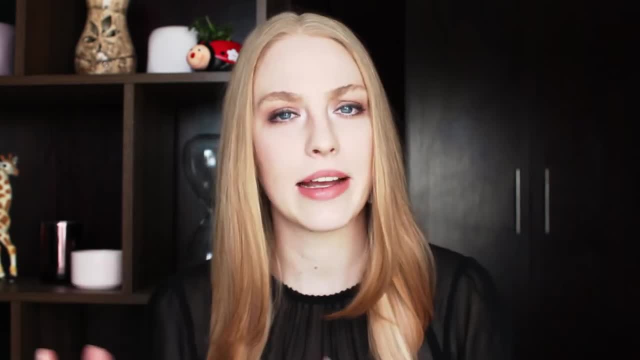 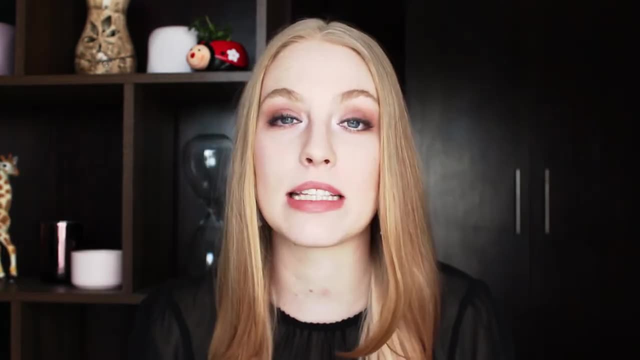 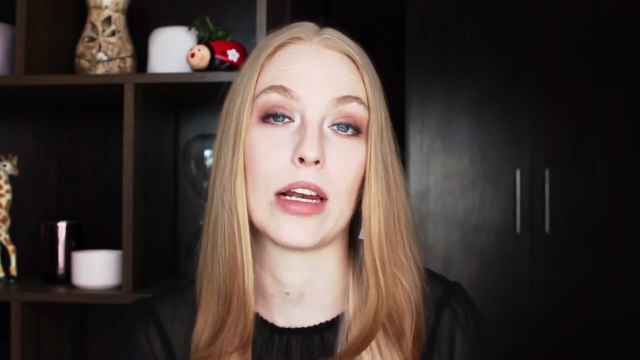 density of housing. Now, remember, density refers to how many people there are within a certain area and remember, for the rest of this video we will be looking at square kilometers. So if there are more people within the square kilometer, we say that that place has a higher population density, or? 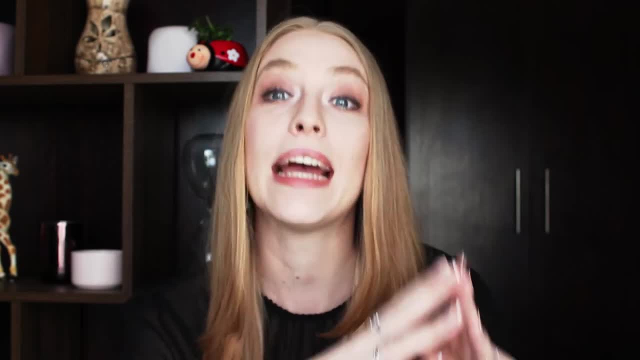 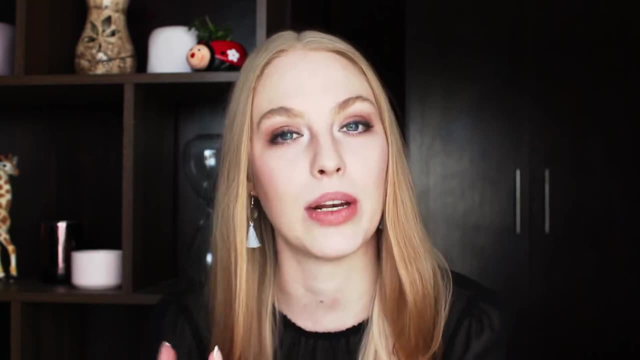 we say that it is a very dense population. If there are very few people within that square kilometer, we say that that population is very low. That means that we have a higher population density. population is very sparse. There is a calculation that goes along with population density and it 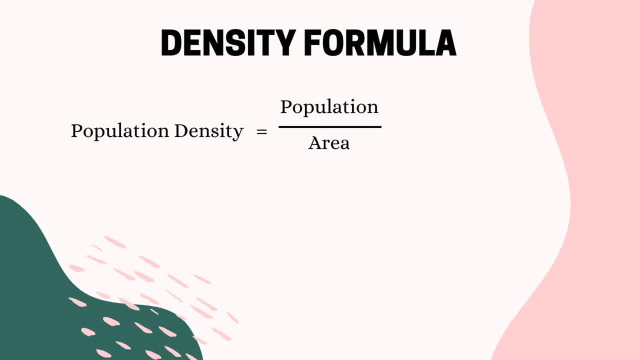 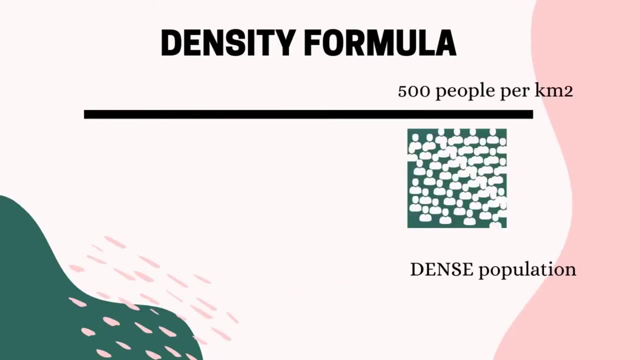 looks like this. Population density equals the total population divided by the area, and now the unit will be people per square kilometer. Obviously, the higher the number is, the more dense this population will be, and the lower the number is, the more sparse this population will be. 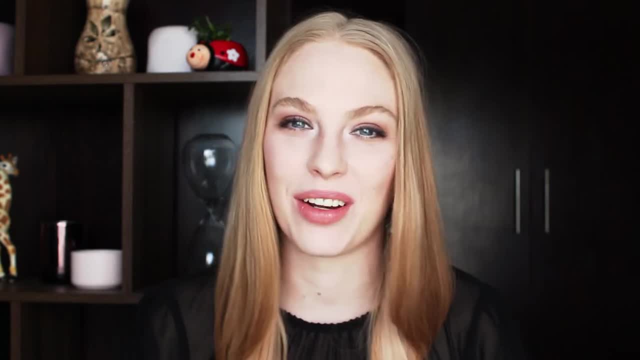 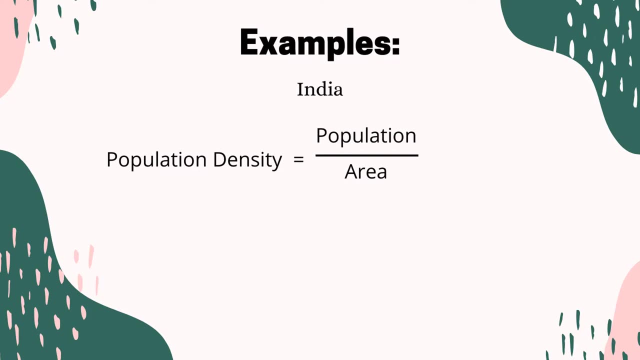 Let's practice some population density calculations. The first country we will look at is India. The latest data that I could get for India in terms of its population size is 1,380,400,385 people, and then we have to divide it by the area, which is 3,287,259.06. 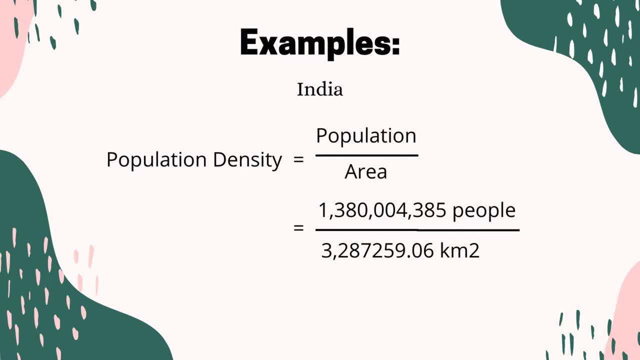 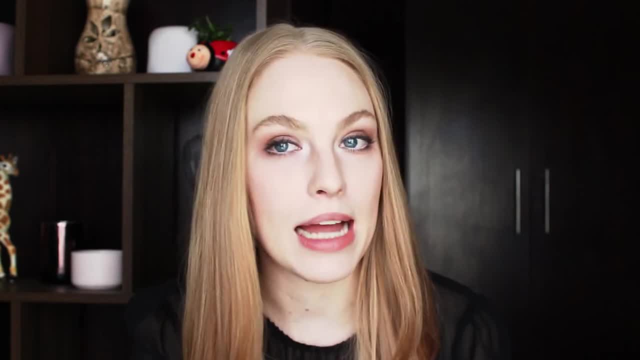 square kilometers. So that's the population density. Let's practice some population density calculations And if we put that in our calculator, we get an answer of 419.80 people per square kilometer. So let's just round that up. Can you imagine within one square kilometer having 420 people? 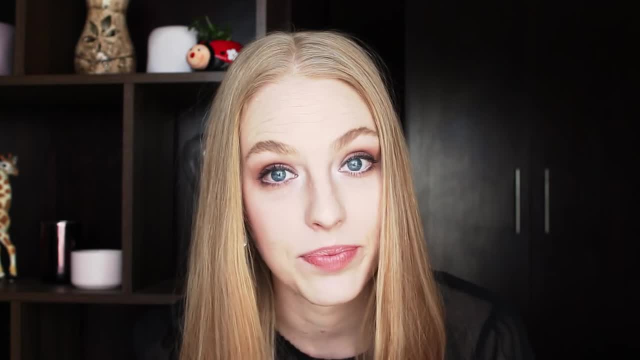 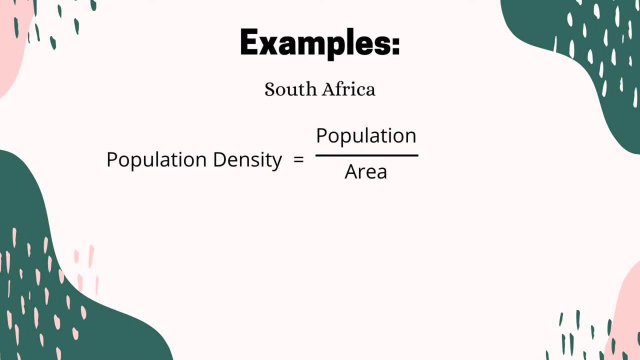 That is the average population density of India. Let's look at another example: South Africa. The latest information I could get on the population of South Africa is 59,308,000 690 people divided by the total area of South Africa, which is 1,213,090 square kilometers. 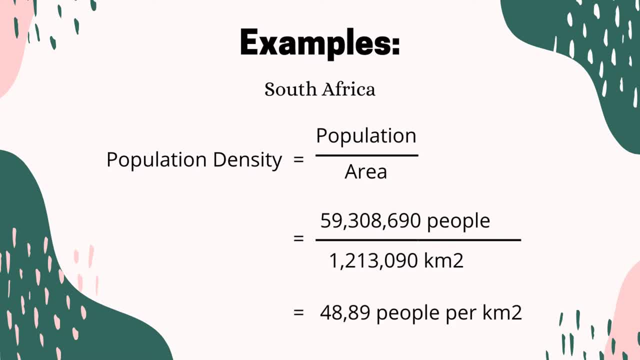 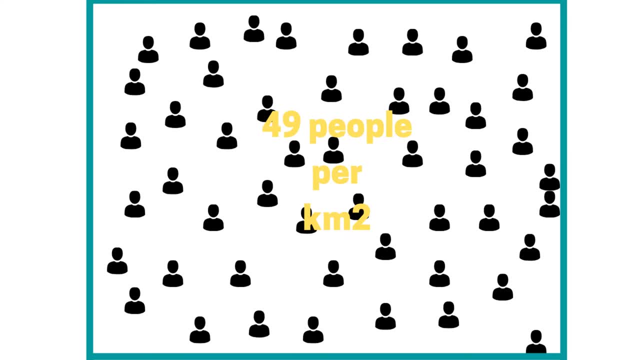 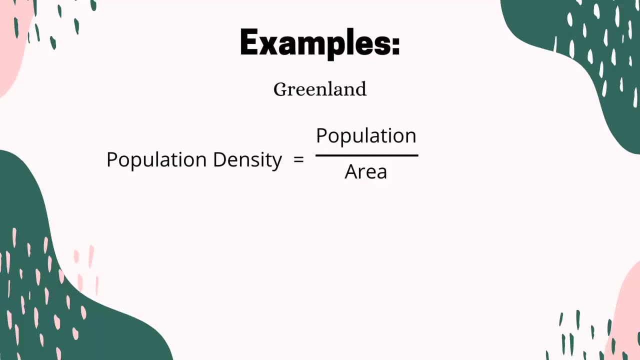 Put that in your calculator and you get 48.89 people per square kilometer. Okay, so let's round it up. That is about 49 people within one square kilometer. Let's do a third example: A country which is very sparsely populated, Greenland. 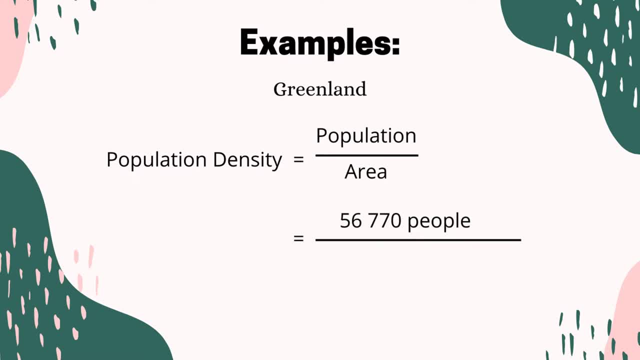 Currently there are about 56,770 people living in Greenland and the total area of this country is 2,166,086 square kilometers, So putting that in our calculator will give us an answer of 0.026 people per square kilometer.